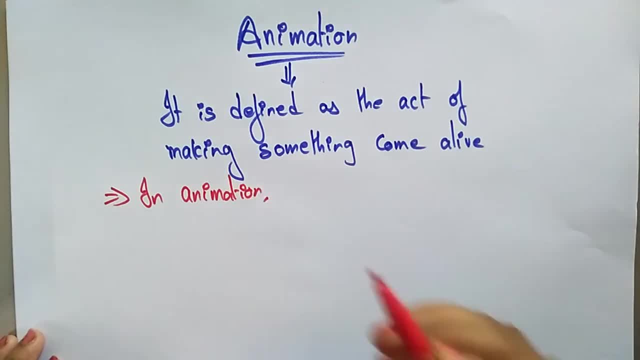 In animation, a series of images, A series, A series of images rapidly change, rapidly change to create an illusion of moment. An illusion of moment, That is an animation, So how you will get it out how the pictures are running. okay, 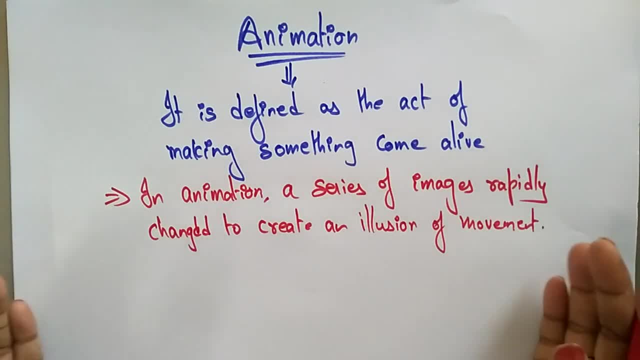 How the pictures are moving. Suppose, if any picture is there, That picture won't. That picture wants to walk on the road, So how this going to be done? Because that is a picture. It actually it doesn't have any life. 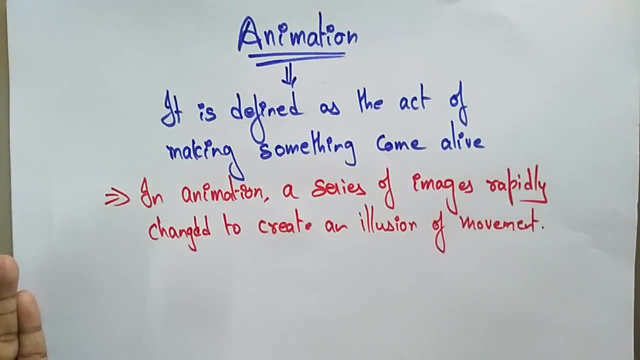 But the picture is moving, okay. Means it is, you're making something alive. How it is possible? Actually, the animation is a series of images. Means the person who is stand here. he wants to walk. okay, He wants to walk. 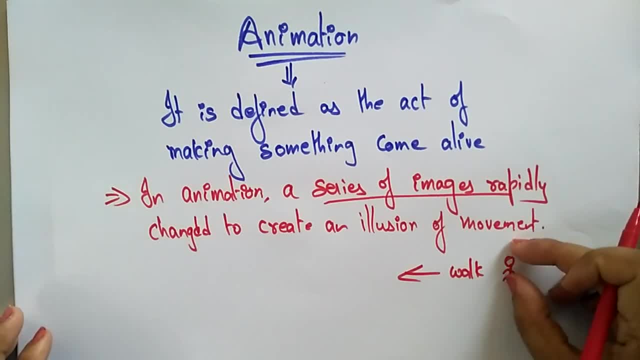 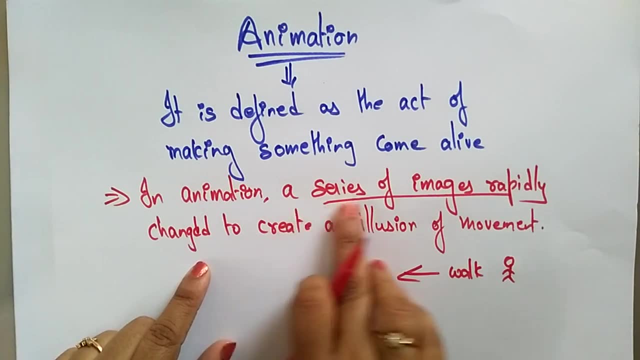 So this is an image, This is an object, This object moving across- Okay, Across on the screen. How it is possible? I am just making a series of images. I am just creating a series of images. okay, The same picture, just like a walking. I am creating a series of images and I am rapidly. 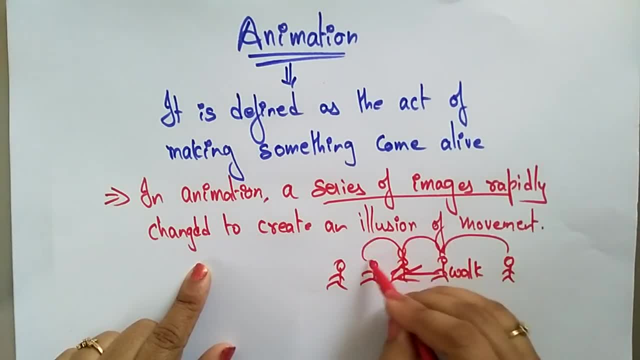 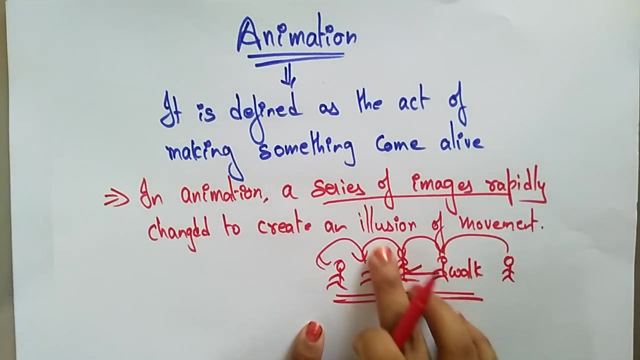 changing. I am just rapidly changing, But it to create an illusion of moment. So I created. the only thing here is I created a series of images, So I am just adding this series of images to the current picture So that the picture is created, an illusion that it is that person is moving. 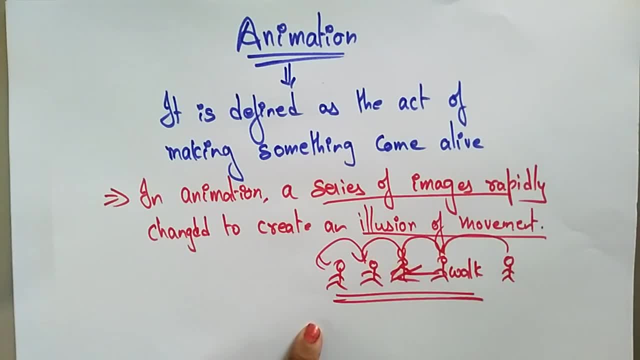 It's just an illusion of moment. That is an animation. So to create an animation you have to make a series of images and you have to make rapidly changes of that image So that it creates an illusion, illusion of moment. So I hope you understand. 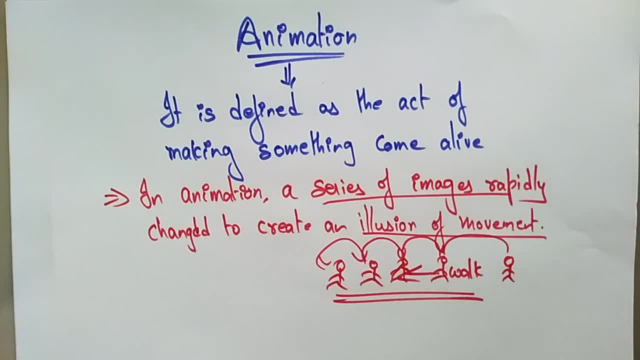 Okay, I hope you understand what exactly the animation is. Animation is defined as the act of making something come alive. Okay, So how this animation will be occur? You are simply, you are just making a series of images, rapidly change it to create an. 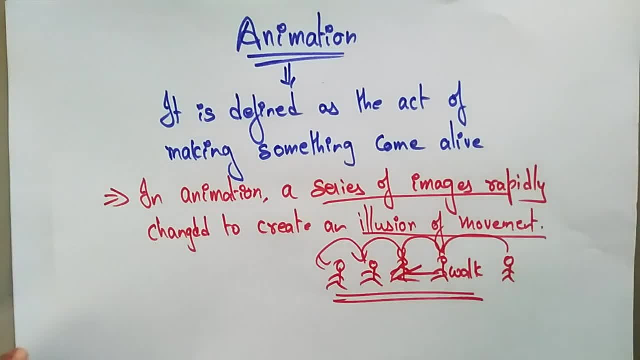 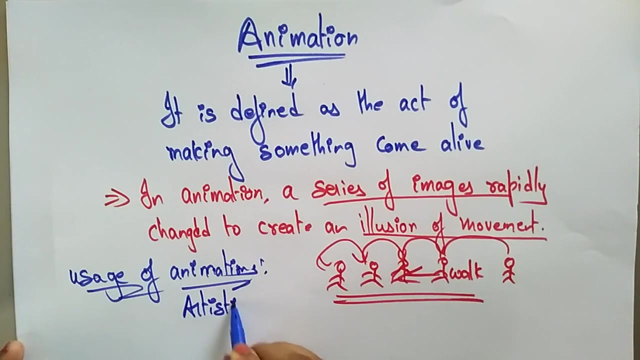 illusion of moment And where this, where we use this animation, So the usage of animations in, so where we use these animations. so I know you know that, In the field of purpose, artistic purpose, or in the field of storytelling, for storytellings. 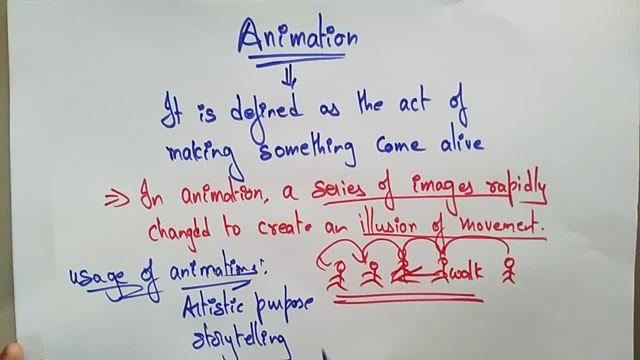 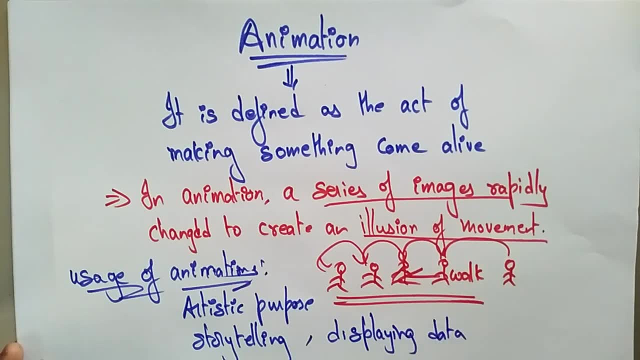 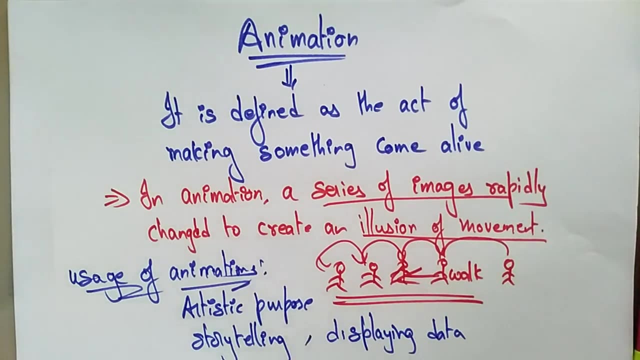 the animated pictures are nowadays very famous and displaying data, in the scientific visualization displaying data and in the instructional purposes. So in this areas we are using these. most of them use the animations. Okay, So now let me explain you the different types of animations. 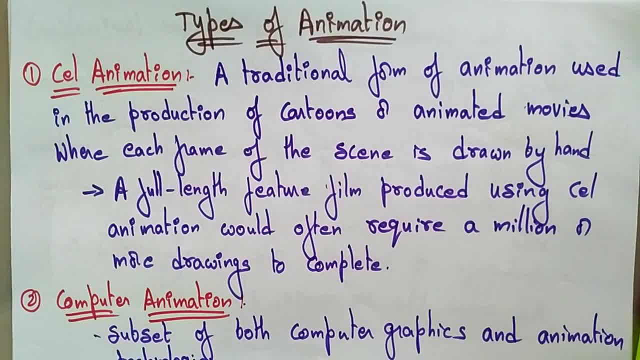 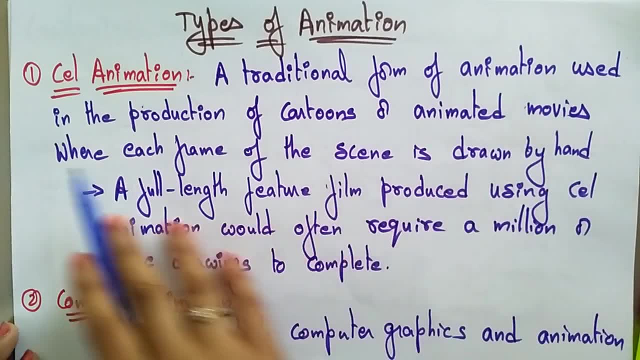 There are different types of animations. In different, different fields, different types of animations will be used. Now let's see what is this? cell animation, a traditional form of animation used in the production of cartoons or animated movies, where each frame of the scene is drawn by. 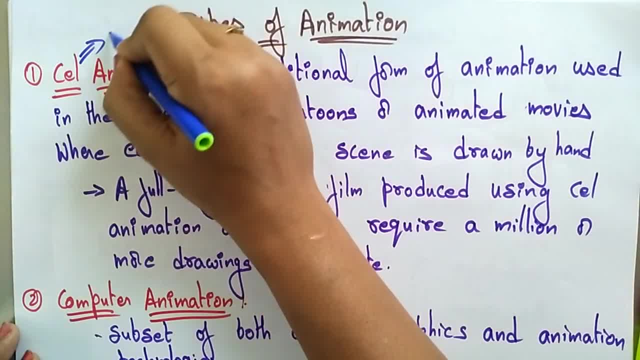 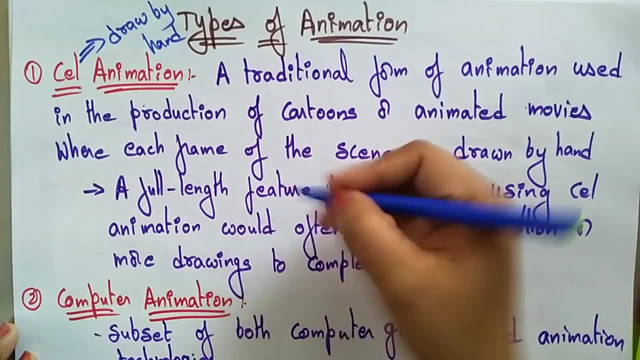 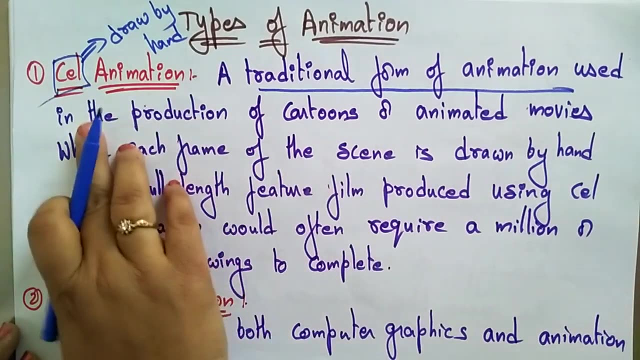 hand. Cell animation means draw by hand, means you are drawing the pictures by hand, means in the paper you are drawing the pictures. So the this you call it as a traditional form of animation. Okay, The cell animation is a traditional form of animation because it is used in the production. 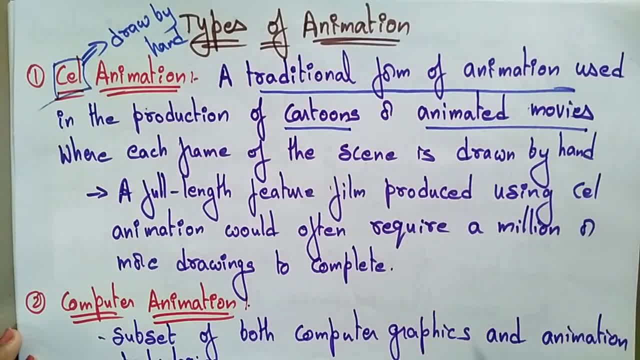 of cartoons or animated movies. So there you are creating a frames of scene in. draw by hand means so many pictures you are drawing and you're making them combine and you're making a picture and a cartoon and animated movie You are going to be created by simply drawing by hand a full length of feature filling produced. 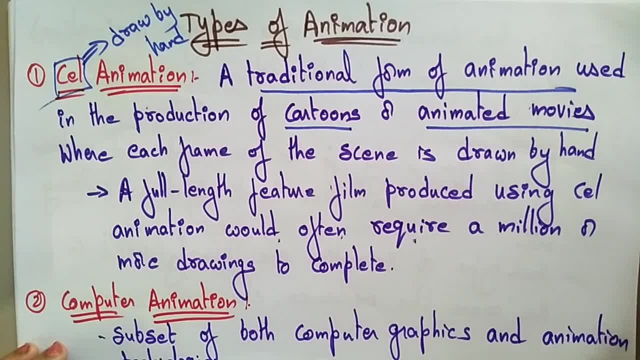 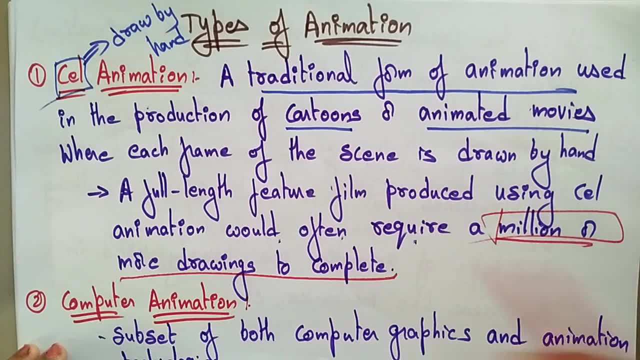 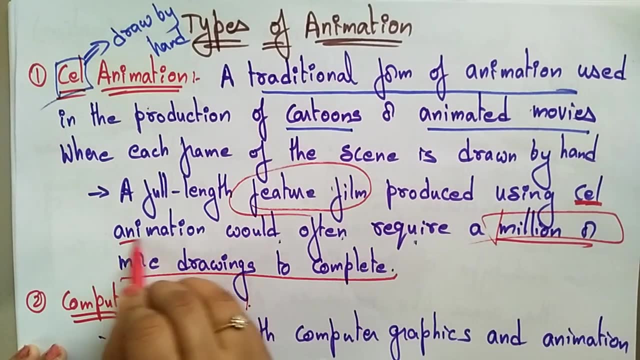 using a cell animation, It would often requires a million or more drawings to complete. If you want to make any a full length of feature filling, okay. if you want to make any full length feature filling by using cell animation, remember that you're using cell animation. 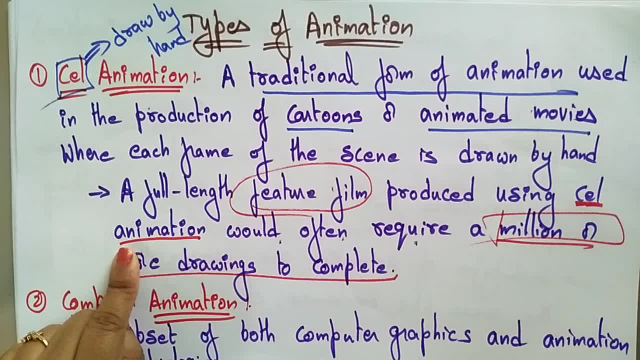 Whenever you're using cell, animation means it's nothing, but you're drawing by hand, So for that you requires a million or more drawings to complete the picture. that much of pictures, Because you need to be drawn in each page. you are going to draw a millions of drawings. 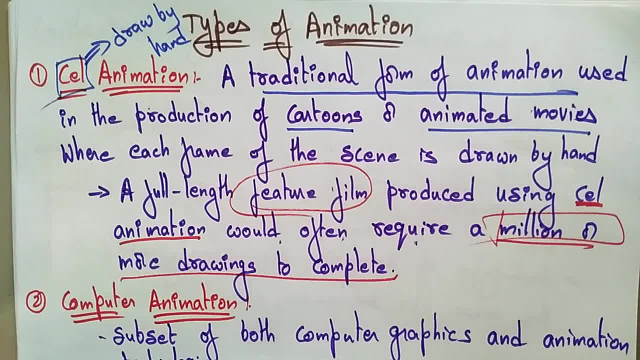 so that a feature film will be completed as a full length film will be completed. It means it's approximately So. the one type of animation is a cell animation. The cell animation is, it's a traditional form of animation, which here each frame can be. 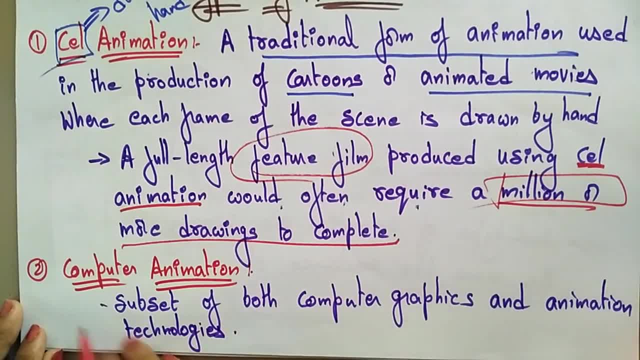 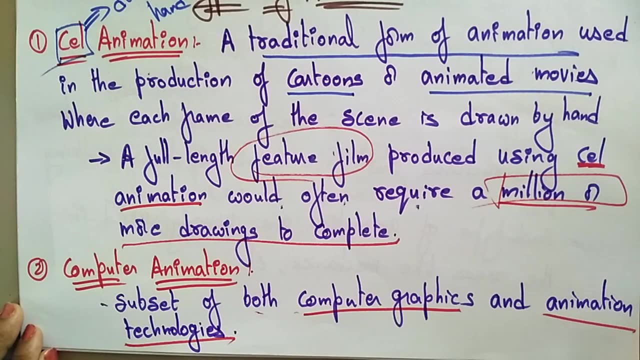 drawn by hand and another type of animation that is a computer animation. So in this computer animation there is no need of drawing the picture by hand. Here we use the computer graphics. it's a subset of both computer graphics and animation technology. Okay, the computer animation it's a combination of computer graphics and, as well as the animation, 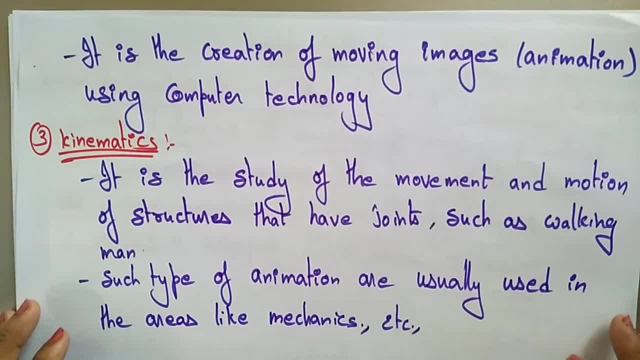 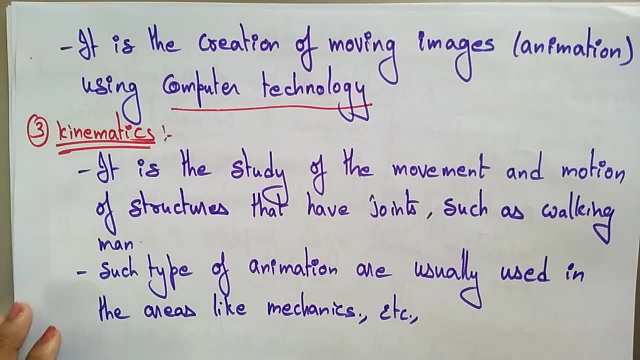 technology. It is a creation of moving images, that is, the animations, using computer technology, So that animations- whatever we are creating, that is, moving images, that will be the animation- will be created By using computer technology. and another type of this animation is the kinematics. 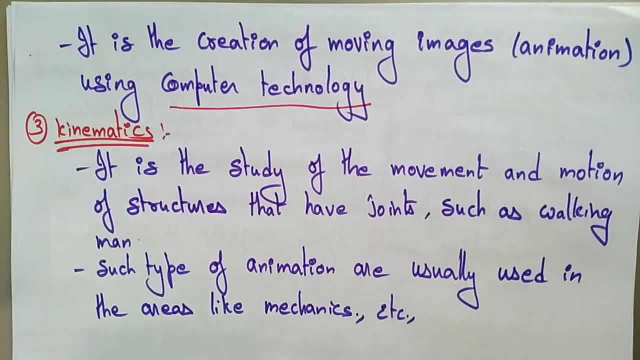 So whenever you heard this name, it's nothing. it's related to the physics, a kinematics. It is a study of movement and motion of the structures. So it's a study of movement and motion, just movement and doing some action of structures. 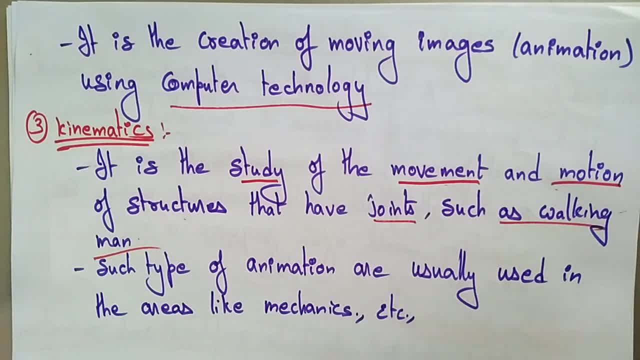 that have joined, such as working a man suppose, if the person wants to work, how he can walk by stride? He can't walk. he has to fold his leg while he's walking. Okay, just like he has to fold his leg and he has to walk. 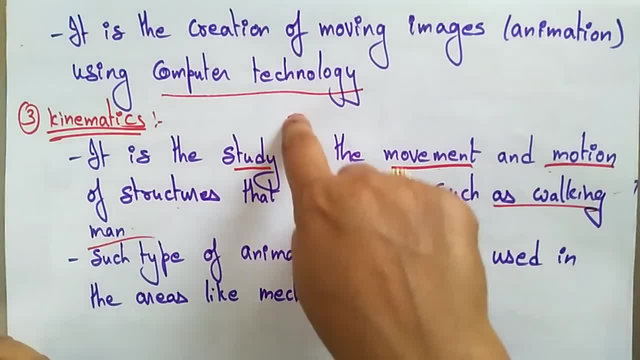 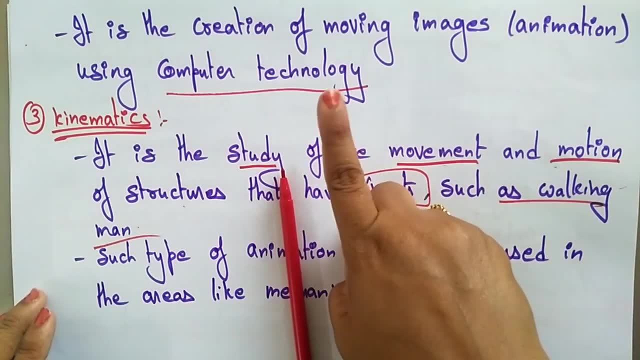 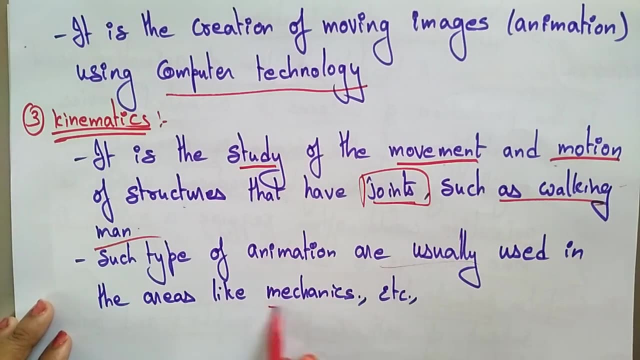 Okay, so further there is a movement should be there and the motion should be there so that it will be work. and here the structure that have a joints- Okay, the leg has a joints and he has to bend like this to work. So such type of animations are usually used in the areas like mechanics. 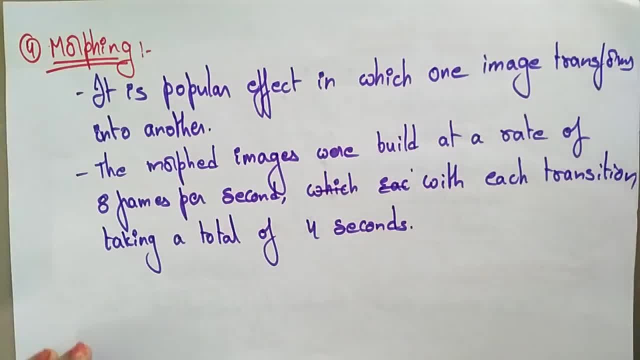 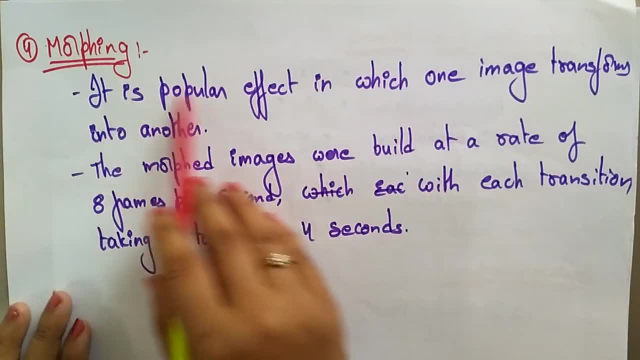 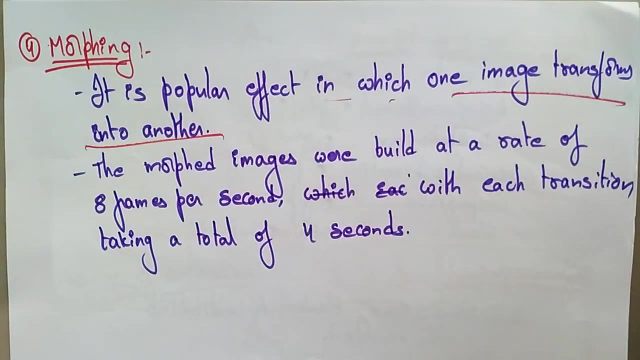 And coming to the another type of animation, So that is a morphing. So I think most of you are familiar with morphing, Because changing the picture, okay, it is a popular effect in which one image transforms into another. So you just simply changing. did you see in the Facebook's nowadays so many links will?